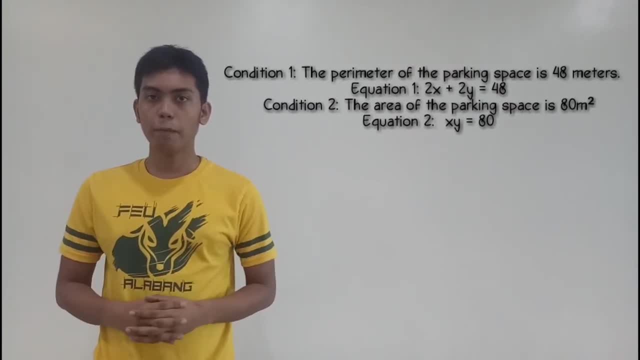 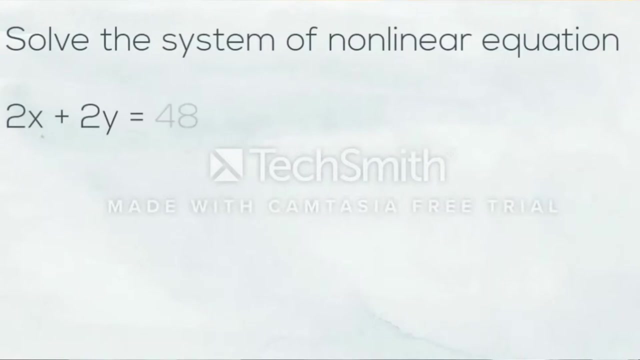 And the equation 2 says that the area of the parking space is 18 meters square. So the equation 2 will be: XY is equal to 18.. So the system of nonlinear equations 2X plus 2Y is equal to 48.. 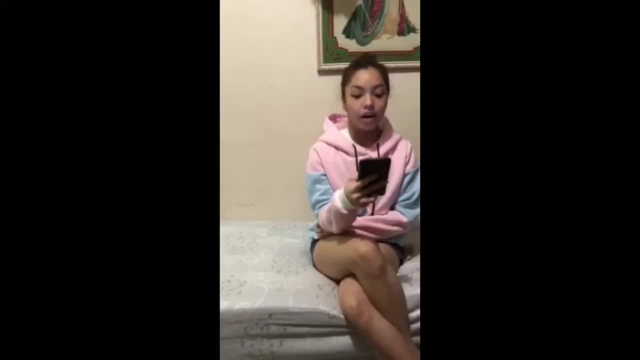 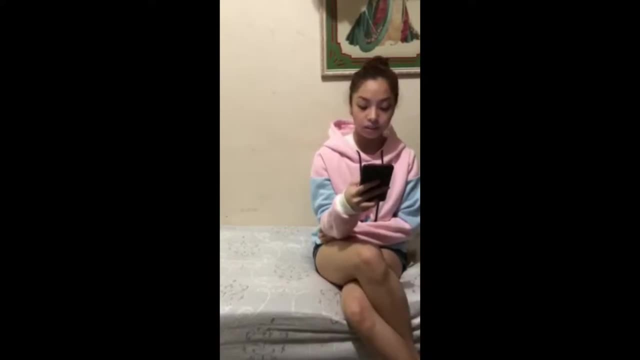 And XY is equal to 18.. What method Can we use to solve this equation? There are three methods of solving this problem: The elimination, comparison and substitution For this equation. we are going to use the substitution method in solving the system of nonlinear equations. 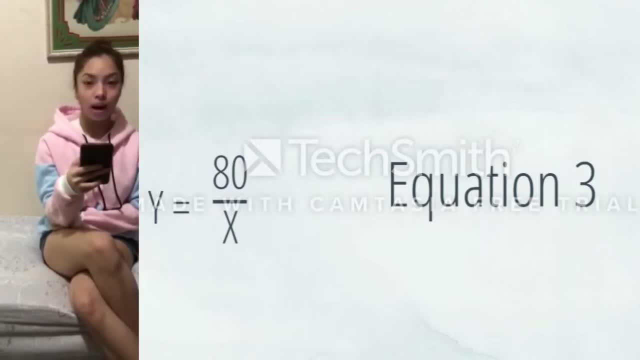 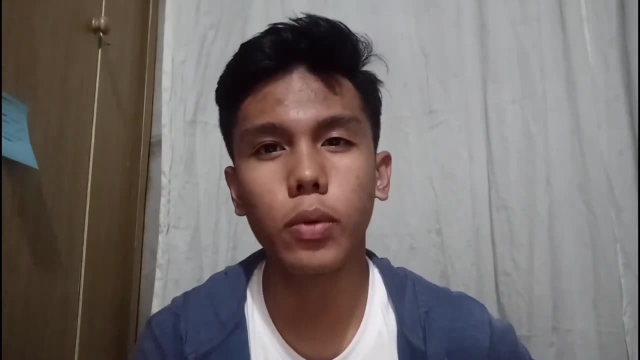 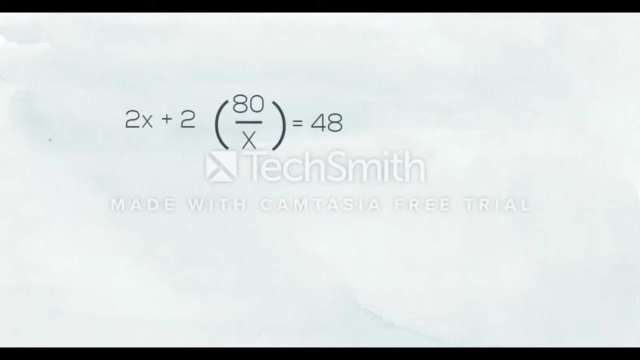 Solve for Y in equation 2.. Y equals 80 over X. Equation 3.. Substitute the value of Y in equation 1 to solve for X: 2X plus 2 over 80 over X is equal to 48.. And 2X plus 160 over X is equal to 48.. 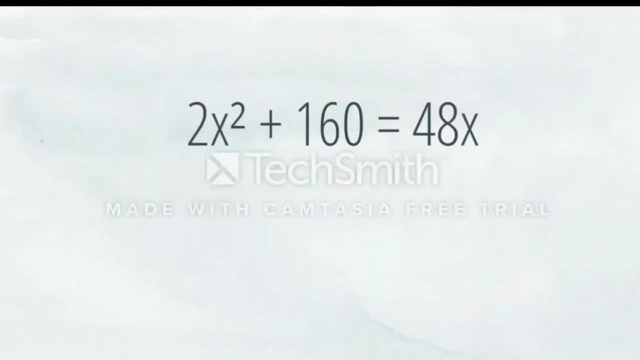 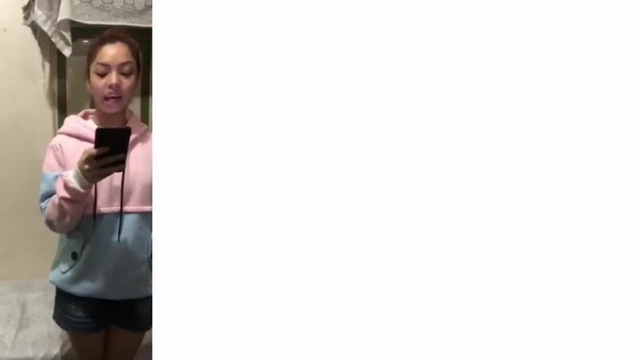 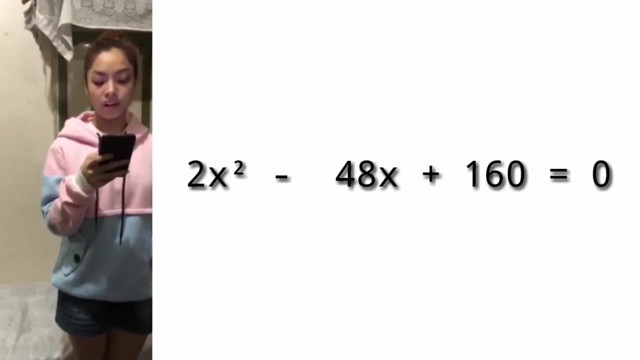 Explain both sides of the equation by X. 2X squared plus 160 is equal to 48X. Set the equation equal to 0.. 2X squared minus 48X plus 160 equals 0.. Factor the left side of the equation. 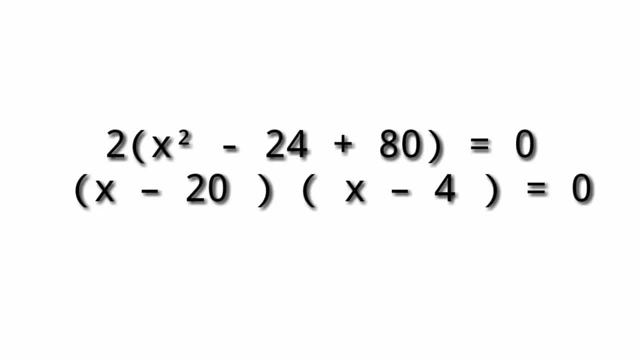 2 multiplied to the quantity of X squared minus 24X plus 80 is equal to 0.. The quantity of X minus 20 and the quantity of X minus 4 is equal to 0.. The quantity of X minus 4 is equal to 0.. 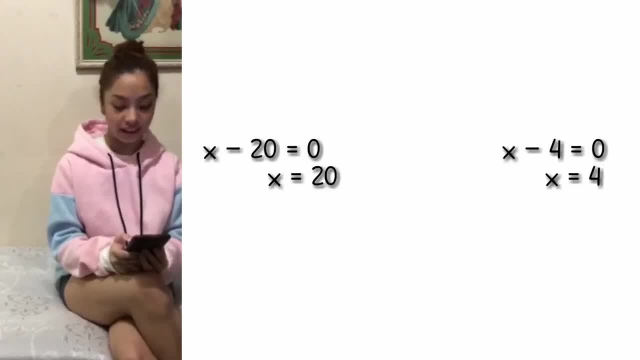 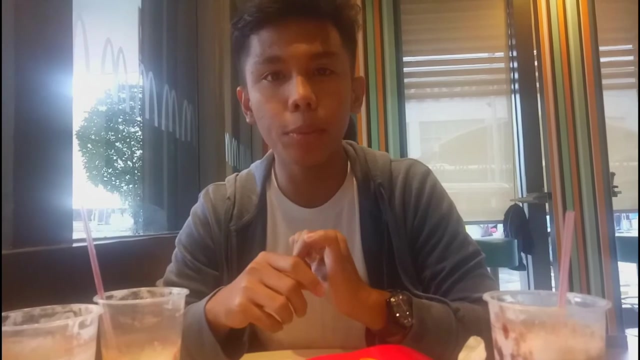 Solve for X using zero-product property: X minus 20 equals 0.. X equals 20.. X minus 4 equals 0.. X equals 4.. Let's just assign this to the parking space. Consider: X is equal to 15.. 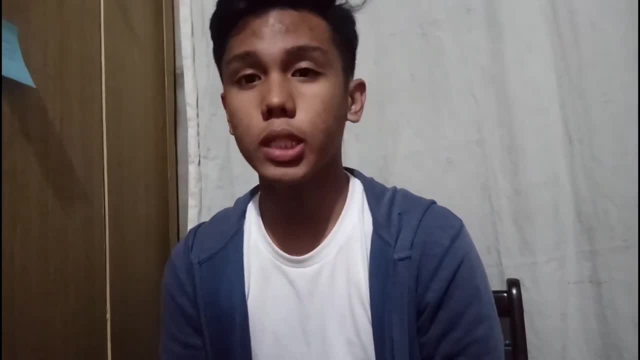 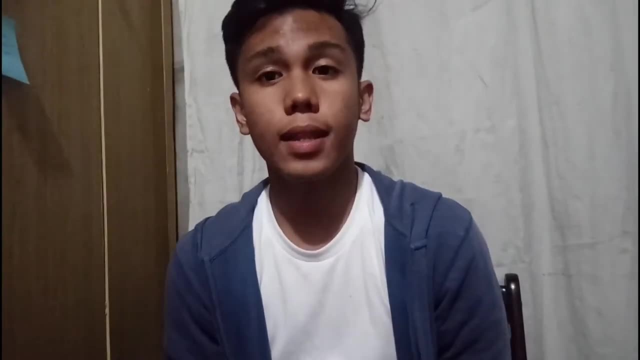 So X is equal to 15 in equation 3.. So Y is equal to 80 over 20.. And Y is equal to 4.. Therefore, the parking space has a length of 20 meters and a width of 4 meters.